often referred to as the continental or contiguous United States, And the state of Alaska has less than a million residents, an incomplete highway system and more natural resources than any place else in the US. So, while Alaska's unique geography provides it with a deep natural 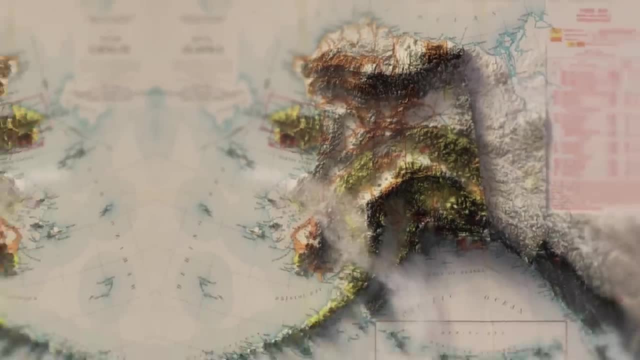 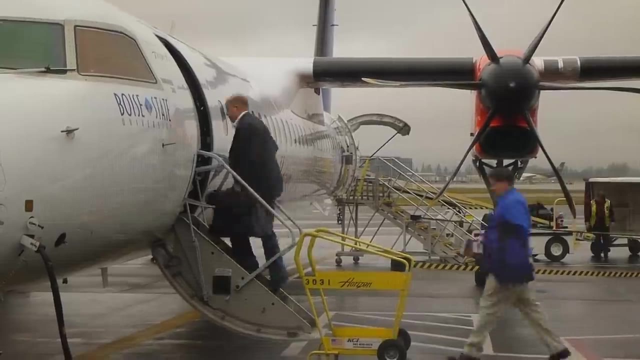 wealth of unthinkable proportions. it also contributes to the state's severe isolation and a lack of city building amenities and modern luxuries there See Alaska can only be reached through air boat or international passage through Canada, And while it's impossible to 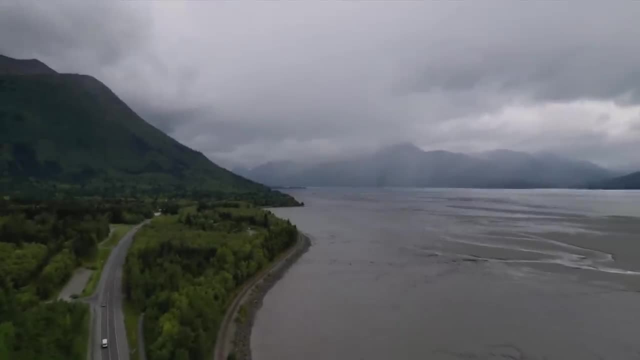 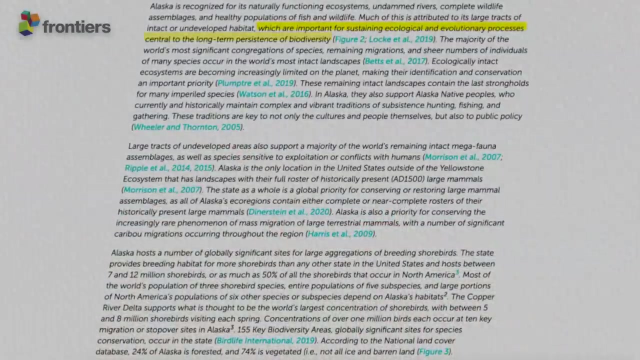 truly describe the awe-inspiring wonder that is Alaskan nature. the words wild, rugged and immense often come first to mind, With Alaska being one of the few remaining naturally wild habitats for animals like polar bears, moose and caribou. 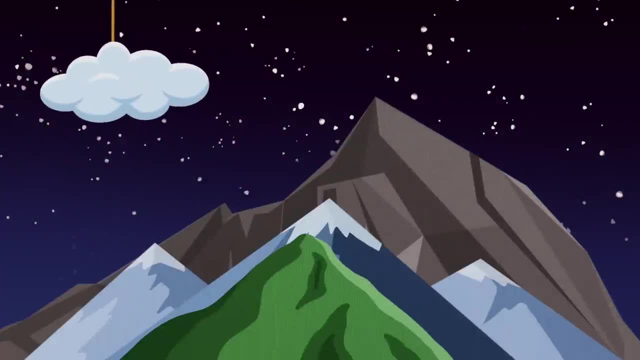 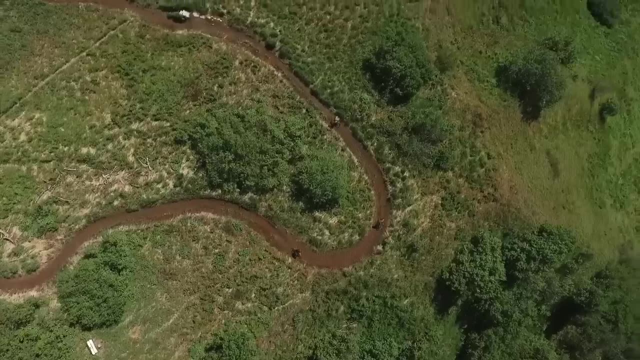 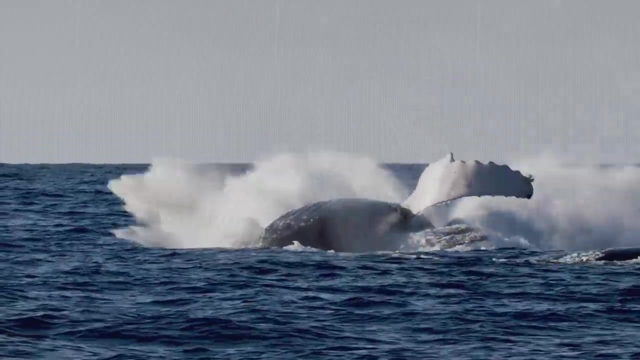 it's also the home of America's first, second and third tallest mountains, including Denali, the highest mountain peak in all of North America. However, Alaska's significant distance to, and separation from the contiguous United States makes life there well, let's just say- complicated. 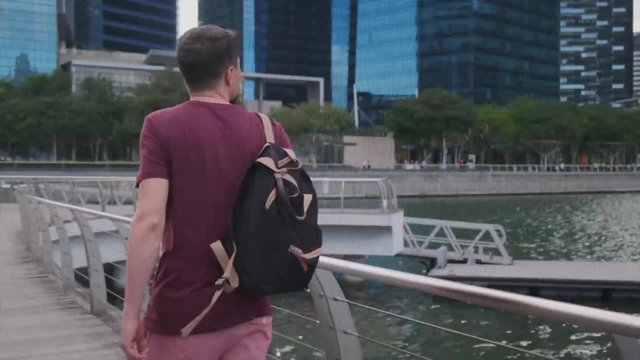 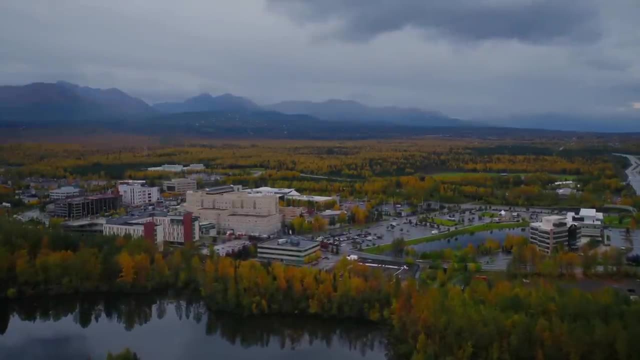 or perhaps even outright difficult, especially when compared to life in traditional US states. As I explain why, that is why life on the Alaskan Peninsula can be very harsh, even for the 730 to 2,000 people that already call it home. I will also be looking at the livability of Alaska's five 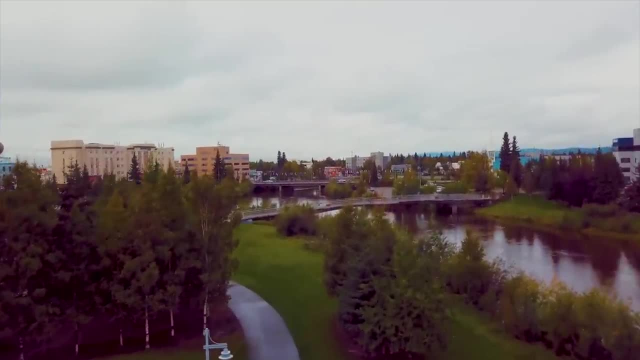 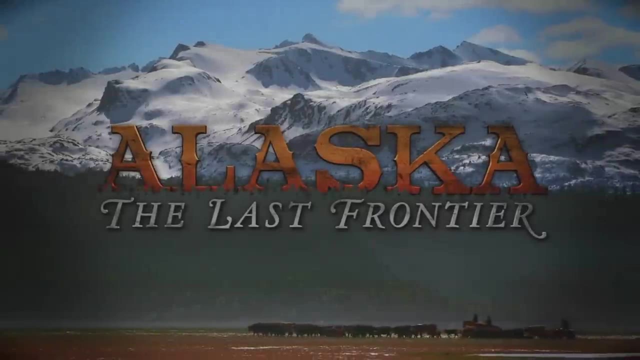 most important cities, breaking down their unique characteristics and why you should, or perhaps shouldn't, consider relocating to the last frontier, And I really think that nickname, the last frontier- says a lot about what Alaska stands for, As Alaska is largely unsettled. 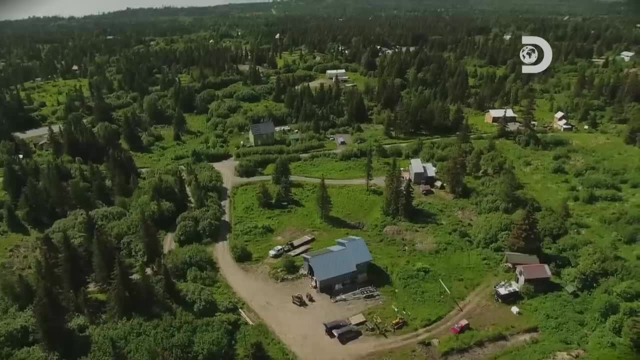 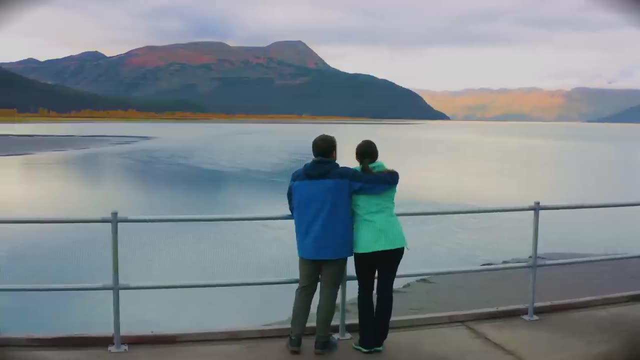 with a few real cities there, serving as a last line of modern settlement, a final barrier between Alaskan society and the wilderness that lies beyond. If you're beginning to wonder if you could even survive Alaska's problematic topography, extremely cold winters and isolation, well, that would be understandable. 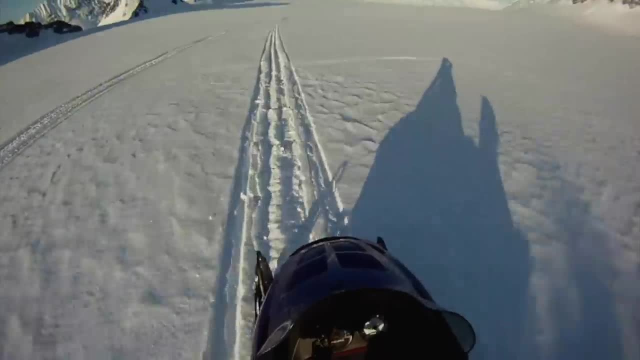 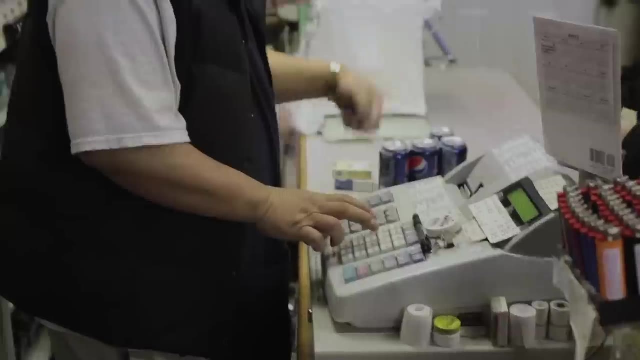 As Alaskan winters are difficult even for lifelong residents, with months of darkness and a polar night that only grows darker as you go further north And small community living in Alaska can be nearly impossible, not only for the difficult terrain and extreme temperatures. 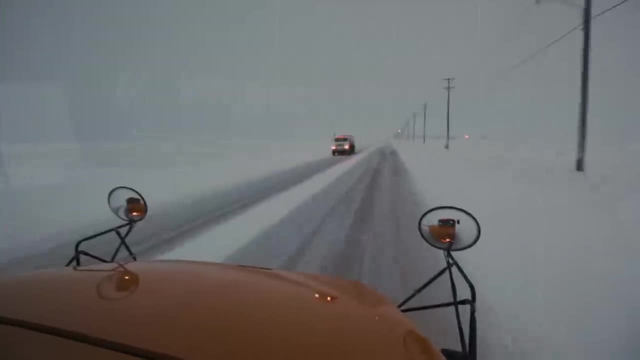 but with several towns completely lacking access to roadway outlets. And yet I would argue that Alaska is a very difficult city to live in and that Alaska is a very difficult city to live in. Alaska's economics and public safety are considerably more concerning for its residents. 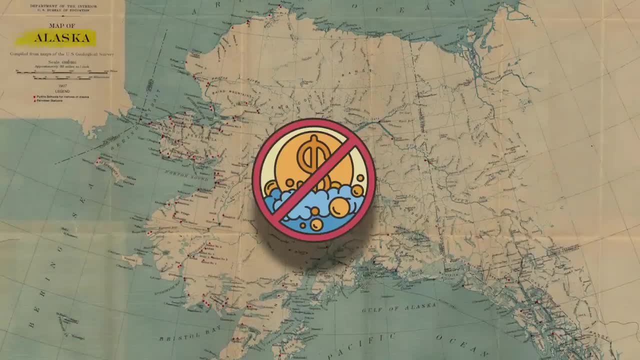 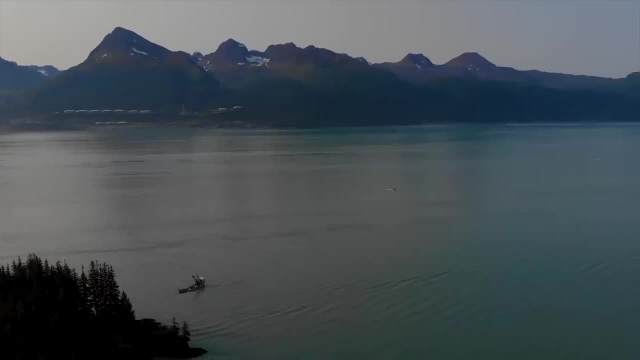 or anyone looking to move there. I will go more in depth on Alaskan economics and safety as I break down the livability of Alaska's most important cities in just a moment, But a more general overview would be that the state has one of the highest crime rates in all of America. 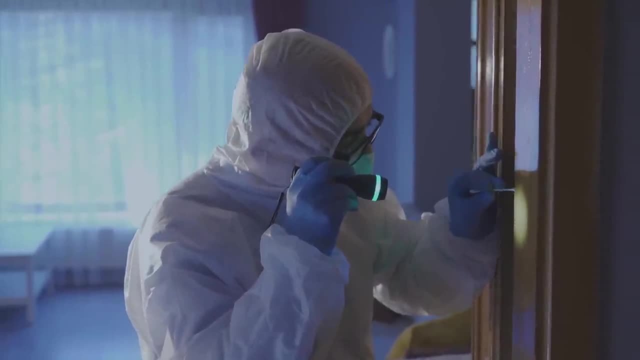 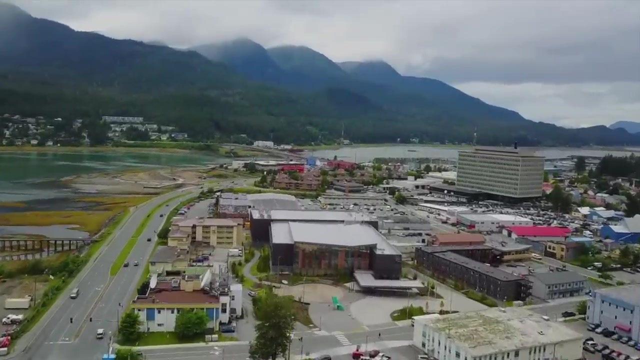 with violent crime being particularly problematic and Alaska having the nation's fifth highest rate of violent crime. The cost of living in Alaska is also nearly 30% higher than the national average, with Alaska being one of the most expensive places to live in the United States. Though, keep in mind, Alaska doesn't levy estate sales or income tax, and median income is very competitive even with the most prosperous of US states. Let's start with Sitka and Ketchikan, the fourth and fifth most populous Alaskan cities. 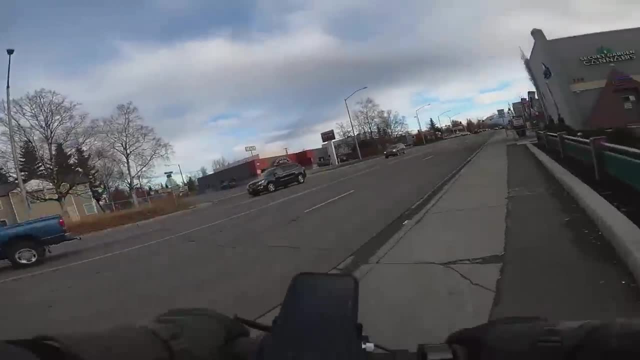 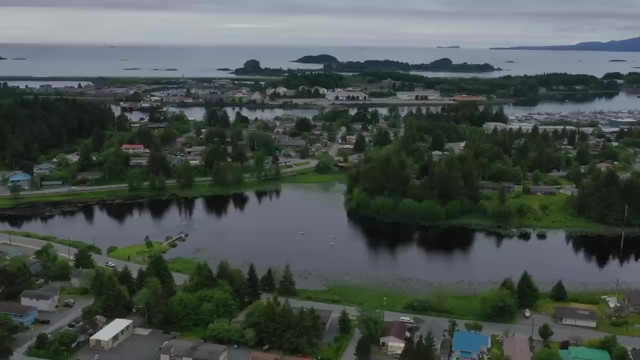 Of course, Kink, Fairview and Wasilla both technically have more residents than Sitka or Ketchikan, but they are part of Metro Anchorage and I wanted to address independent Alaskan cities here. And Sitka, located in southeastern Alaska, is a real city, A very small city with just 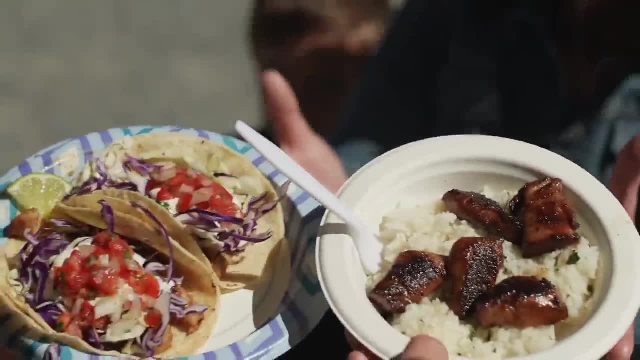 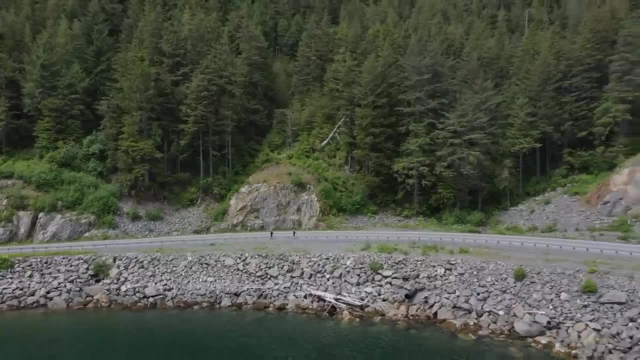 over 8,000 residents, but a legitimate little city nonetheless. Sitka is also an expensive city, though, with a cost of living that's about 40% higher than the national average. Ketchikan is also located in southeastern Alaska, but while it's a bit smaller than Sitka, 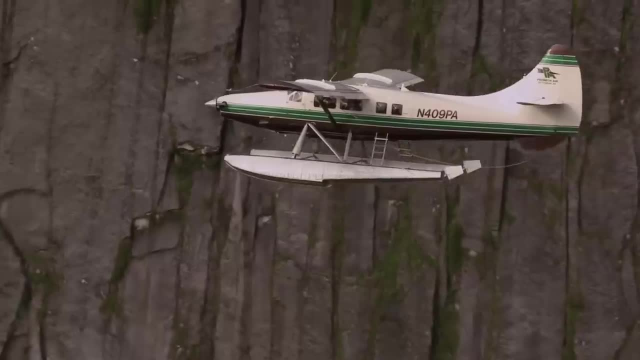 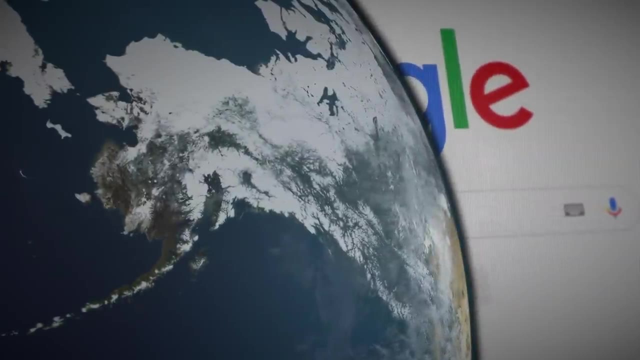 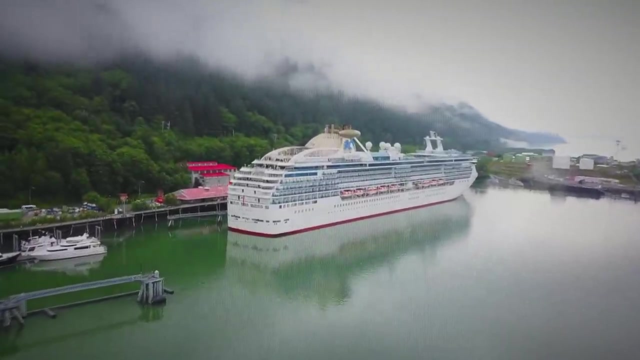 it's arguably more important as Ketchikan serves as an essential hub for the state's fishing economy. Then again, the story of Alaska revolves mostly around its three biggest cities: Juneau, Fairbanks and Anchorage. Juneau is the third largest city in the state of Alaska, despite it having just under 32,000. 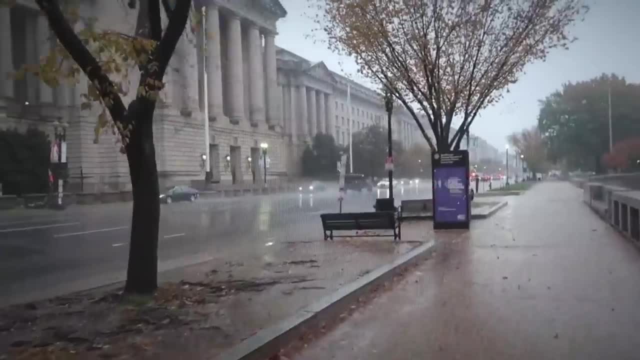 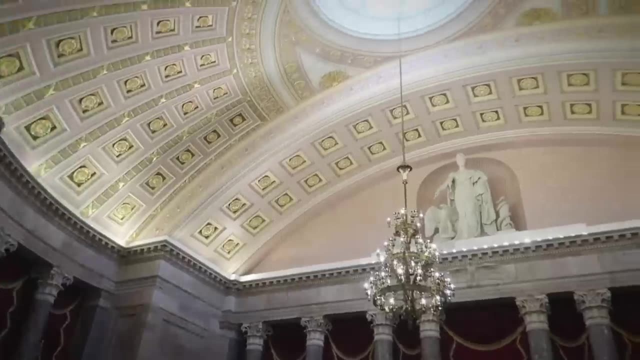 residents and a slightly declining population. Juneau is mostly known for being the capital of Alaska, also located in the southeastern portion of the state, though it can't be reached even by other southeastern cities without a boat or plane, something that I think really outlines. 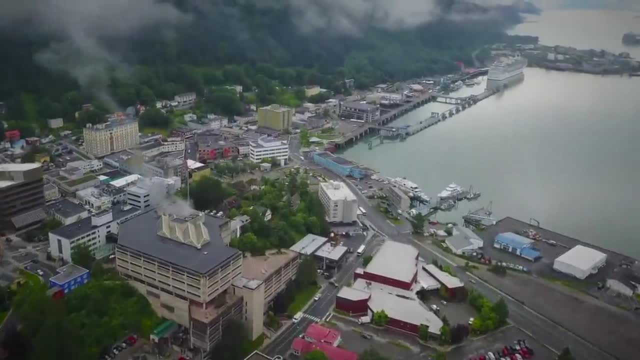 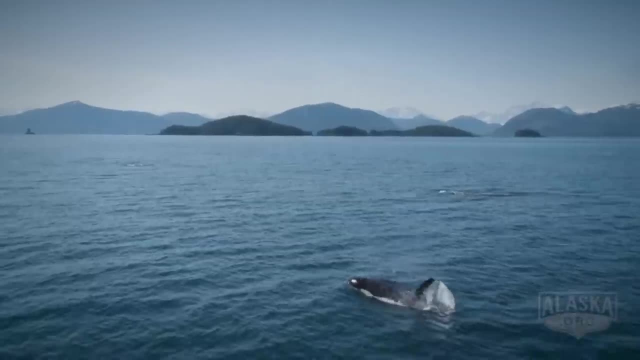 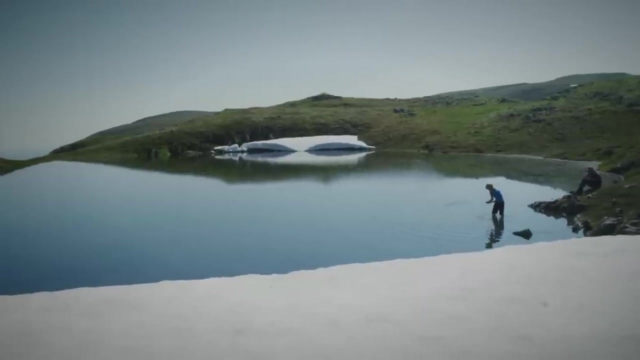 Alaska's staggering size and remoteness. Being the state capital of Alaska, Juneau has a thriving economy with significant employment in government, tourism and fishing. It's known for its natural beauty, surrounded by scenic ocean views and tall mountains. Juneau has the lowest crime rate of Alaska's three big cities and a